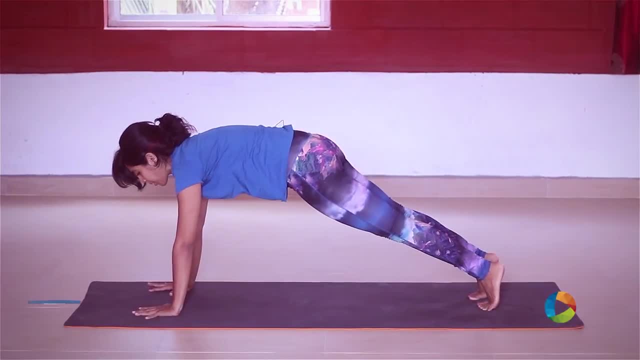 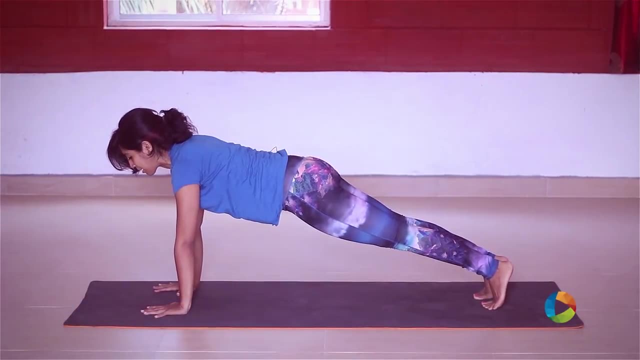 drop your hips. That's really bad because you'll hurt your lower back. So always pull through your belly and make sure the body is in a straight line. Roll the shoulders and keep the body really nice and long and engage your thigh muscles. So roll your shoulders. 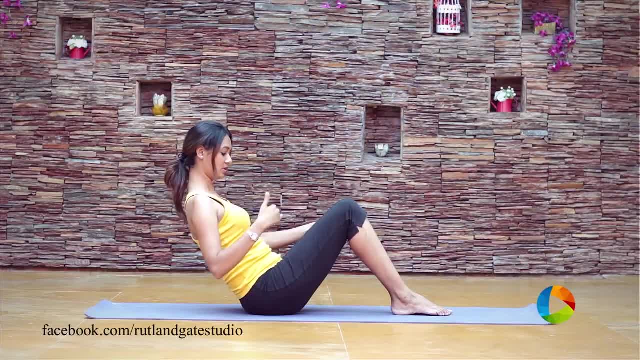 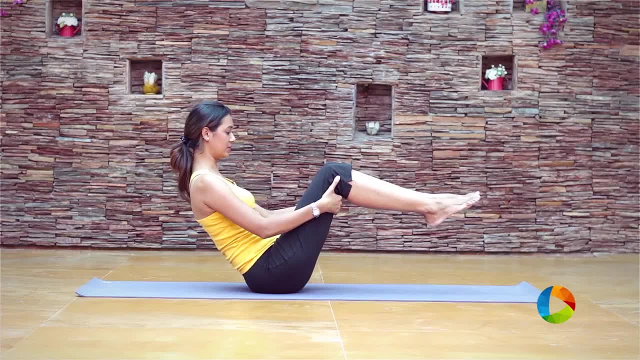 back and slowly lean all the way back, just like this, So keeping your back strong and nice and sturdy. Inhale, lift your legs all the way up and slowly release your arms to the sides of your body and hold the posture, not your breath. Remember to breathe. 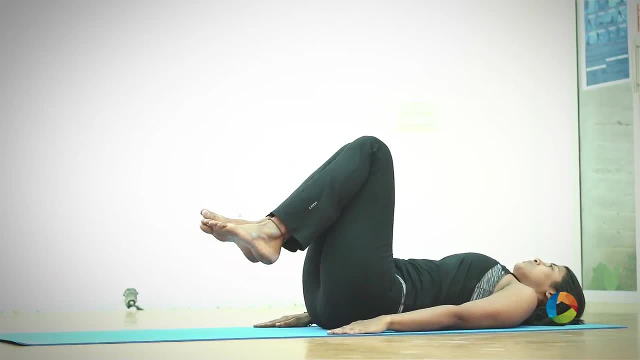 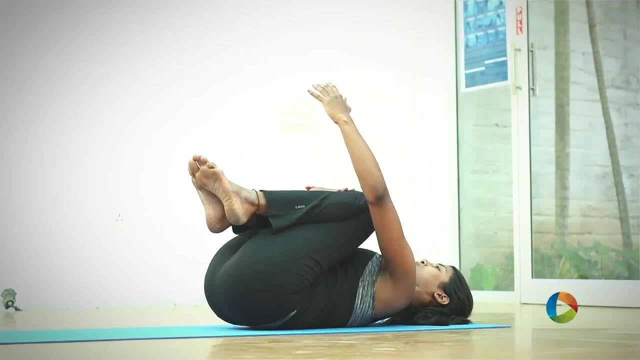 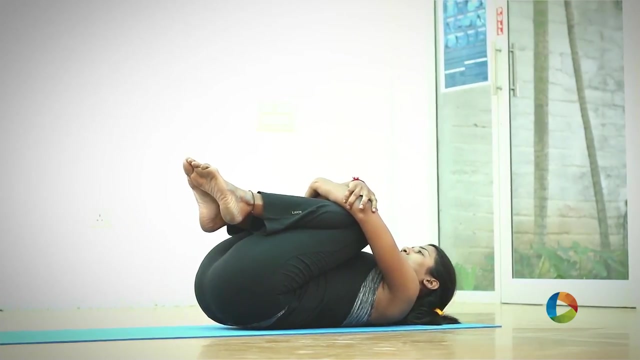 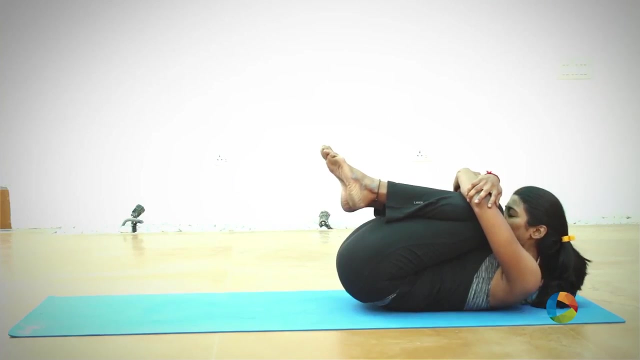 Gently take both the knees towards your chest. Interlock your hands. If you want more squeezing of your abdomen, you can hold both the sides of your elbow. Pull the navel inside as you exhale. Try taking the chin towards the knee. Don't take your forehead to the knee Then. 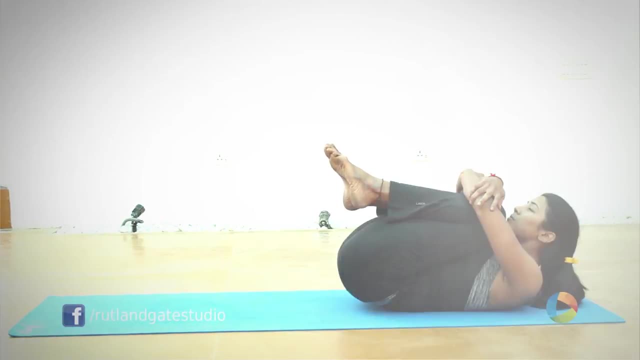 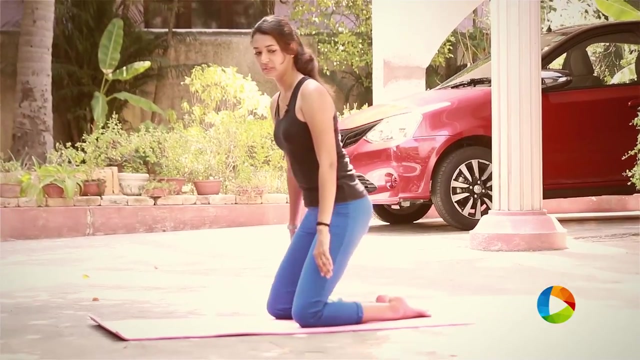 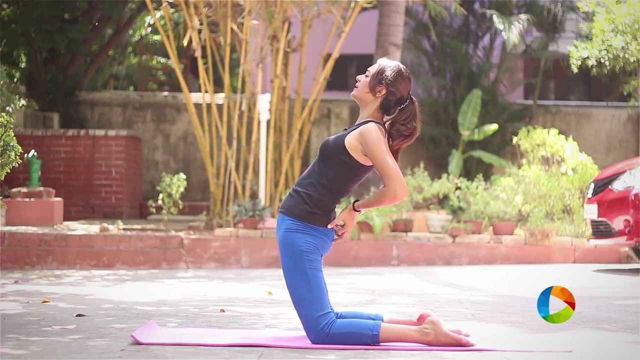 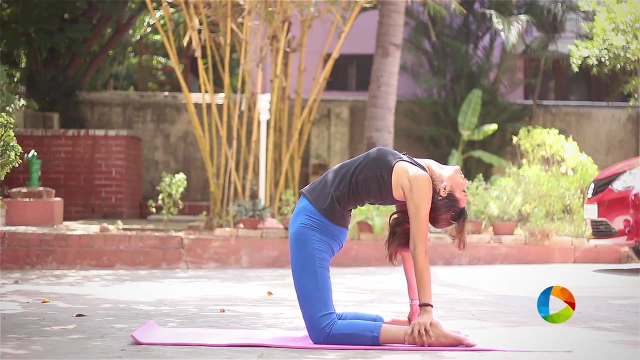 you'll be hurting your neck. So begin by sitting in Vajrasana And what you want to do is basically stand on to your knees and widen your legs. really nice. So inhale, exhale, pushing your hips forward and slowly bringing your arms to your ankles and arch back. 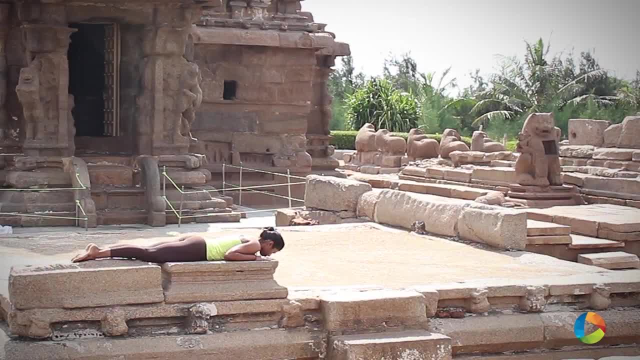 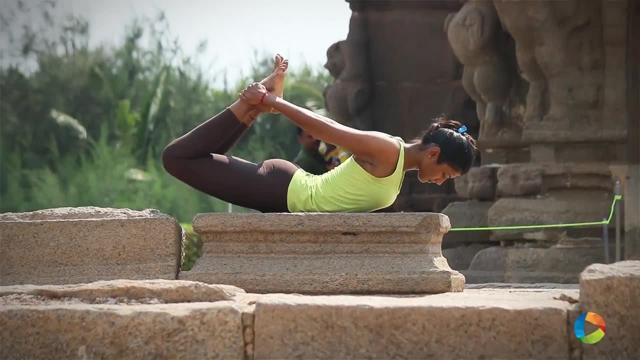 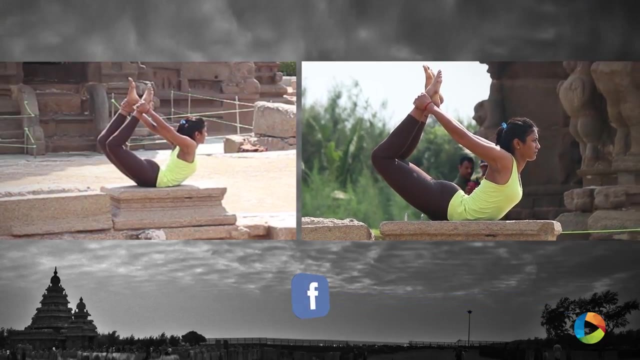 First, lie down on your stomach. Exhale, bend your knees And hold the ankles with your hands Wide. inhaling, raise the thighs, head and chest as high as possible. Try to maintain the weight of your body on the lower abdomen. Join the ankles, look upward and breathe normally. 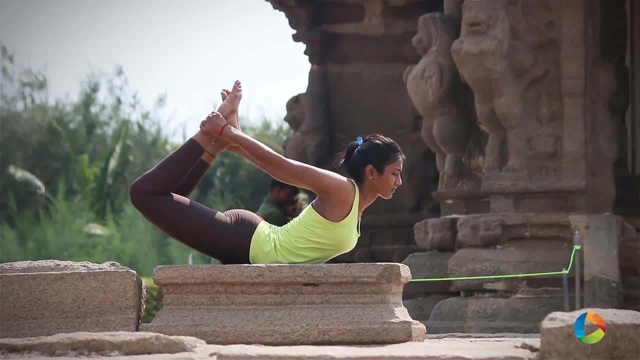 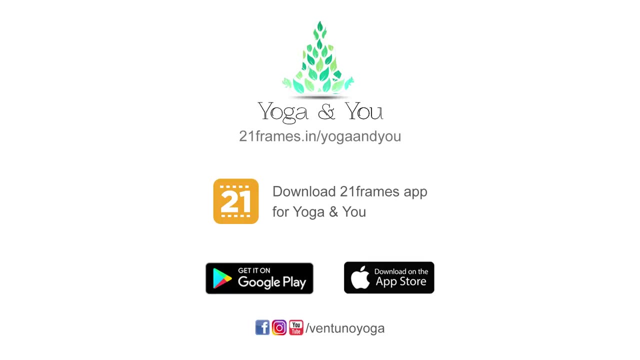 Maintain this position as long as you can hold and slowly come back to the original position. Subtitles by the Amaraorg community.